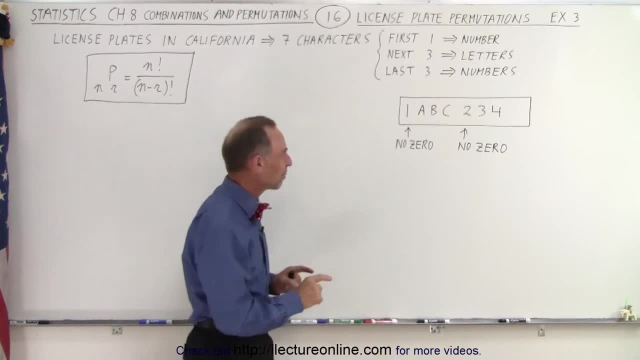 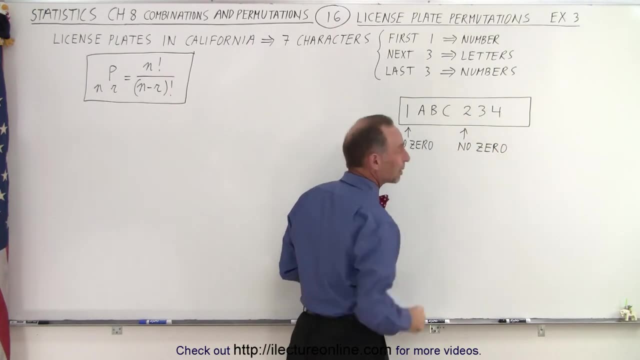 characters were numbers again, And if I remember right- because I don't ever remember seeing it- that this first character cannot be a zero, or this first number cannot be a zero and the leading of the three numbers cannot be a zero either, It turns out this scheme was: 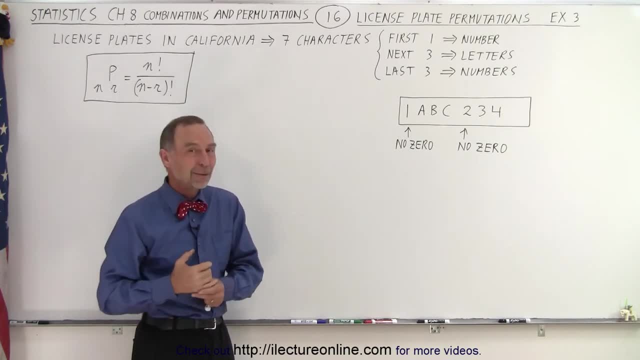 good for a long time, but we ran out of license plate permutations and we had to go to a different scheme and we'll show you what that new scheme is. But let's first calculate how many different permutations there are with this kind of scheme and why did we run out. Okay, let's try this. 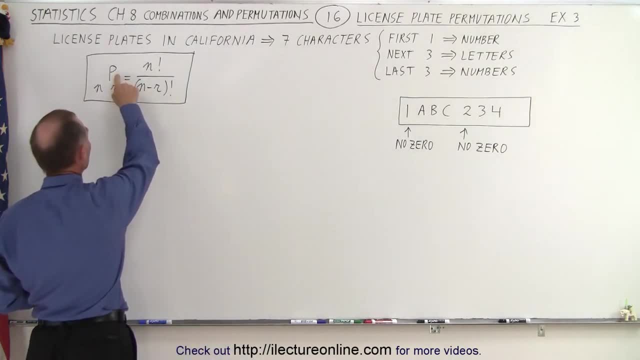 so again we use the same equation: The number of permutations of n and r. N is the number of letters or cab's numbers. This streets says N square. That's the number of letters or cab's numbers, characters we're going to have. r, of course, is the number that we're dealing with in this case. we'll 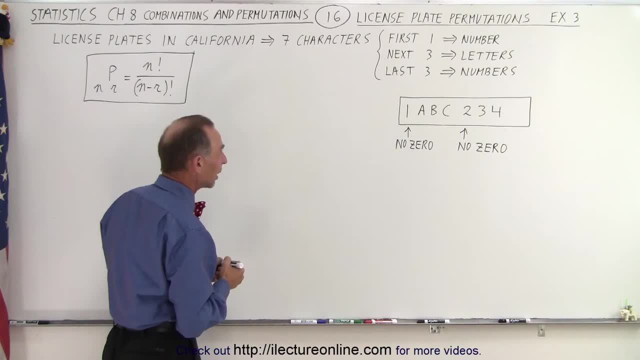 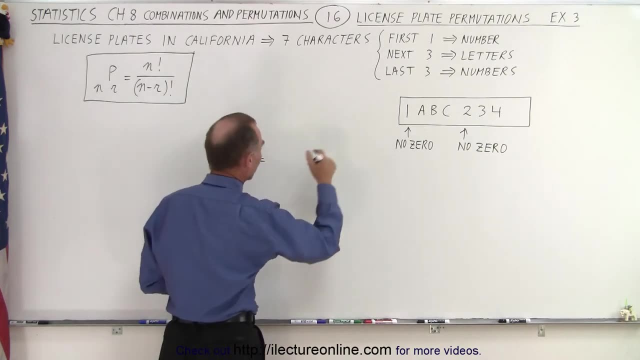 have to take it one at a time, and so the following will then become the number of permutations. so the number of permutations is equal to for the first one, it's going to be p. there's only nine possibilities, if we ignore the one at the zero, and there's only one letter to be picked, and so 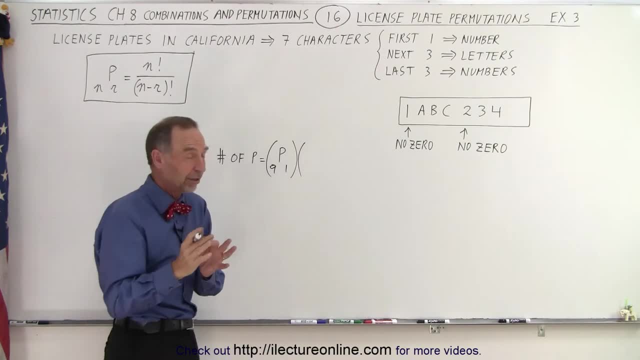 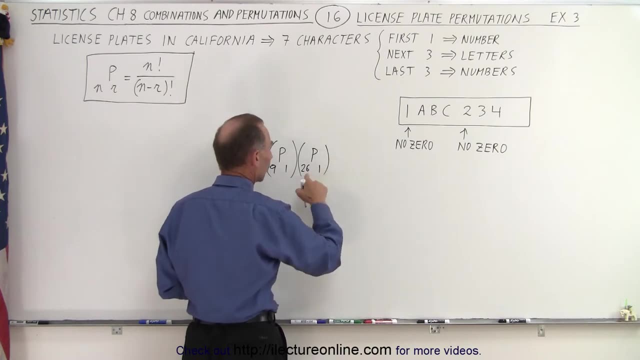 we're going to multiply that times the next three, but we have to take it one at a time. so it would be p, that would be 26 and 1, because there's 26 different letters and all of them are permissible. so we have three of those: 26 and 1, 26 and 1, and then we have three more numbers, but for the first 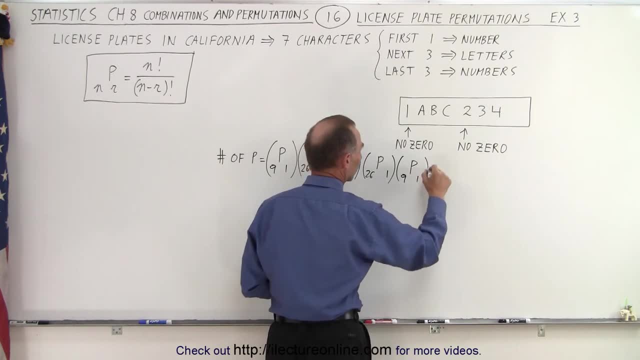 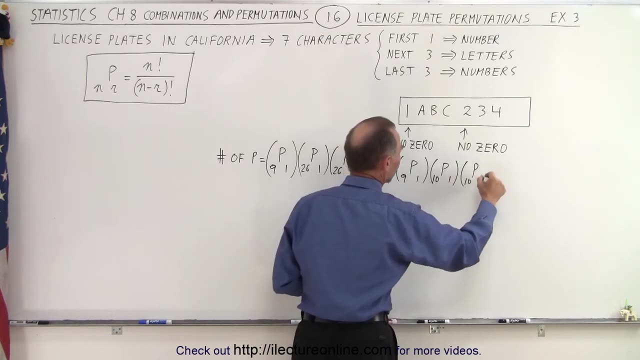 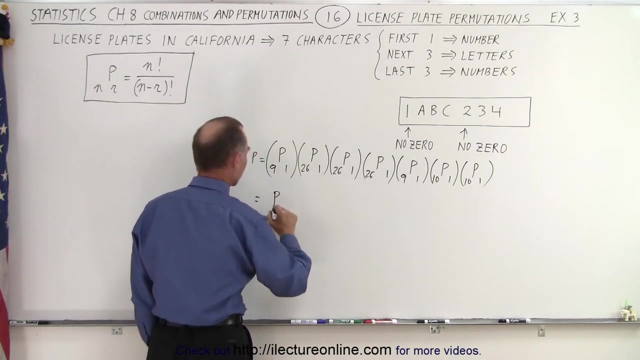 number. there's only nine possibilities because we have to ignore zero, but for the next two we can have 10 numbers, you and so that's what the equation is going to look like, and so, simplified, we could say that this is equal to. we have three of these, so p 26: 1 to the third power. we have two of those. 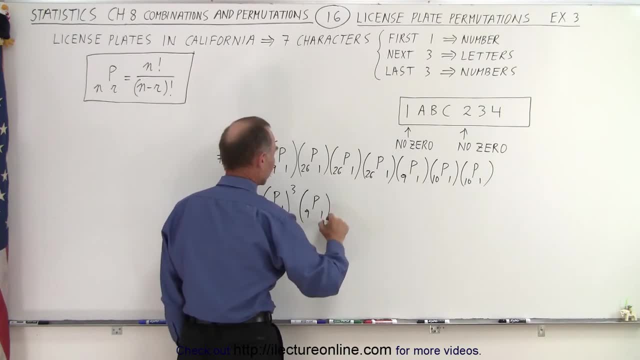 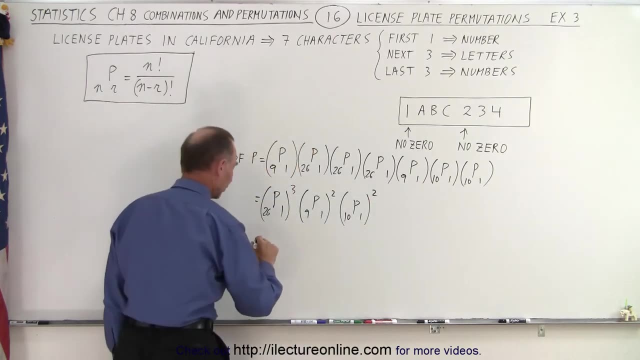 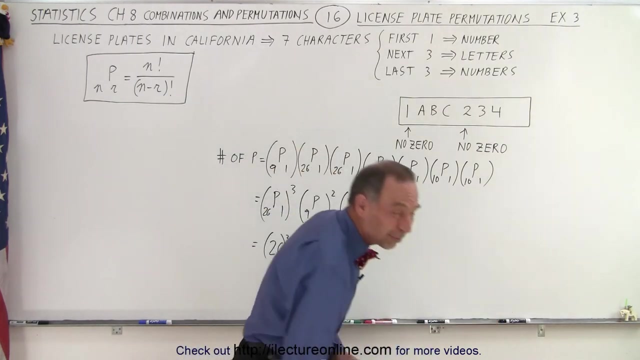 so that would be p 9 to the second power, and then we have two of those, which is p 10 and 1 to the second power. all right, so this becomes equal to 26 cubed- I'll put parentheses around it- times 9 squared. times 10 squared. so how many different permutations are there for license plates? 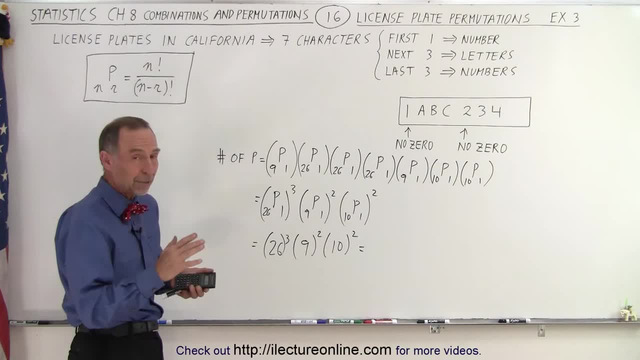 in California using the scheme. that's been good for a long time now. in the older days there were only six characters on the license plate and of course in the very old days there's fewer than that, but that has been kind of the standard, probably for the last 30, 40 years or so, if I. 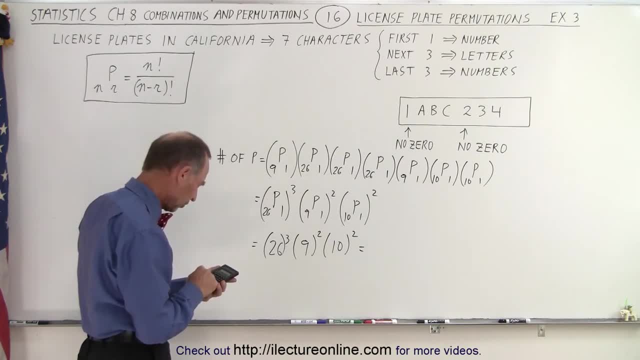 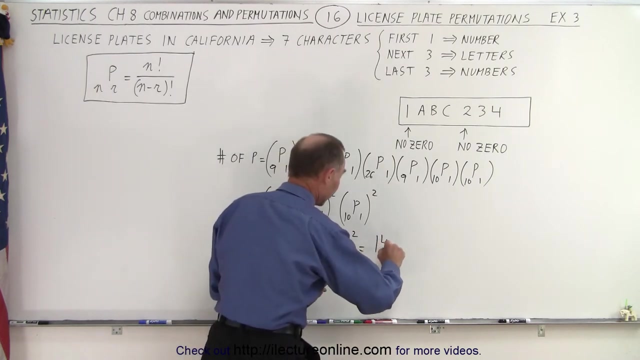 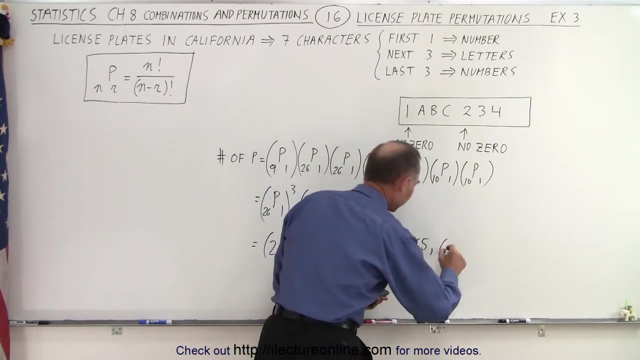 remember right. so that gives us 26, raised to the third power, times 9, squared times 10, squared times 9 squared, which is 81, times 10 squared, which is 100, and let's see here: wow, well, that gave us a total of a hundred and forty two million three hundred and sixty five thousand six hundred. 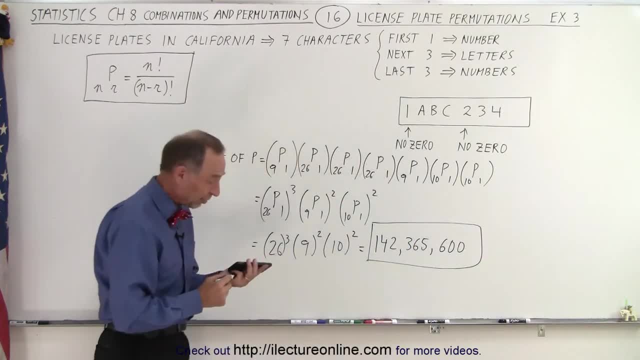 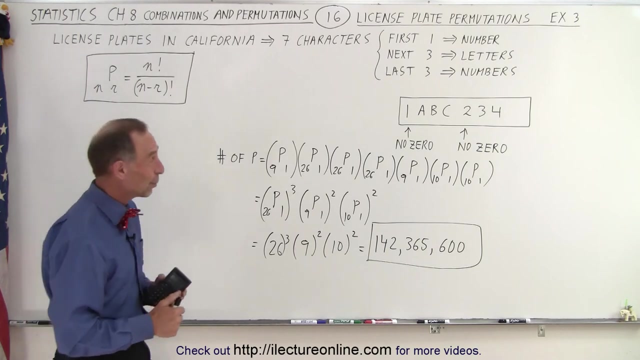 different license plates, and for a population of California being somewhere around forty plus million or so, you would think that should last us for a very long time. but it didn't. we ran out and we had to go to a different scheme. well, what was the different scheme? well, the very first character can now also be a letter, and so that will add a whole number. 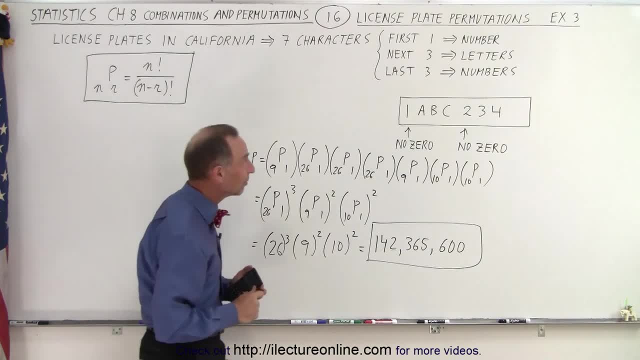 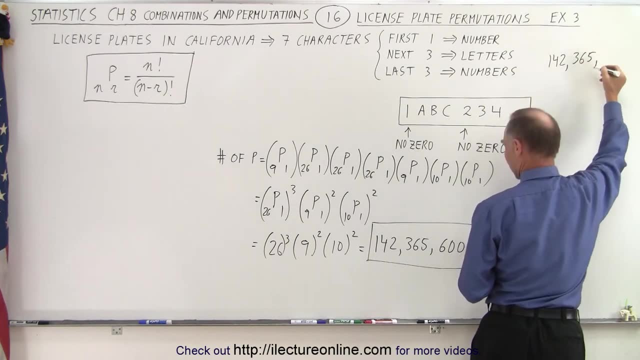 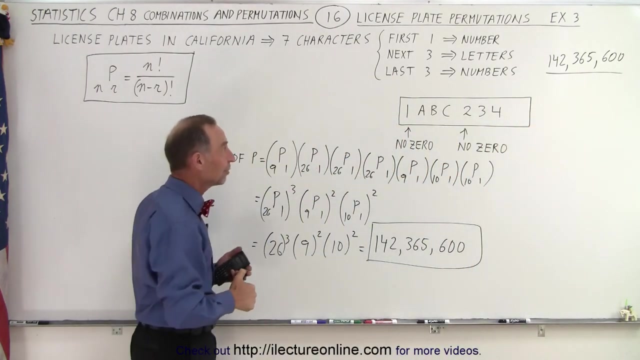 additional permutations. so let's keep that number handy somewhere. so we're going to write that one down. one hundred and forty two million three hundred and sixty five thousand six hundred. and let's say you're asked how many more permutations are there for license plates? and let's say you're asked how many more permutations you would have now if you can also allow a letter. 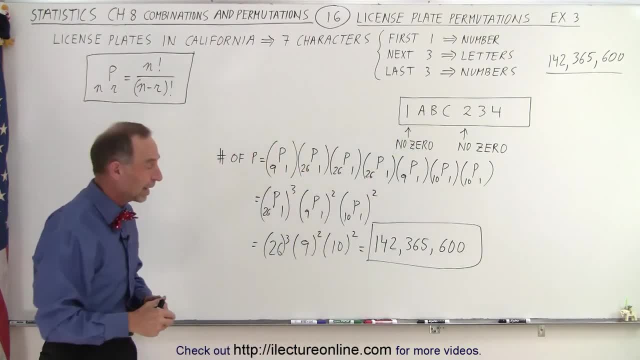 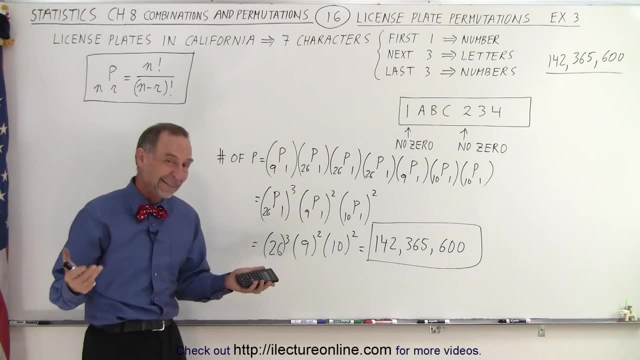 to exist in the front instead of just a number from one to nine. all right, let's go ahead and do that on our next video, and then you can see how much that changes, and we can then guess how many more years we can go with just seven characters on our license plate, until we either have to change the 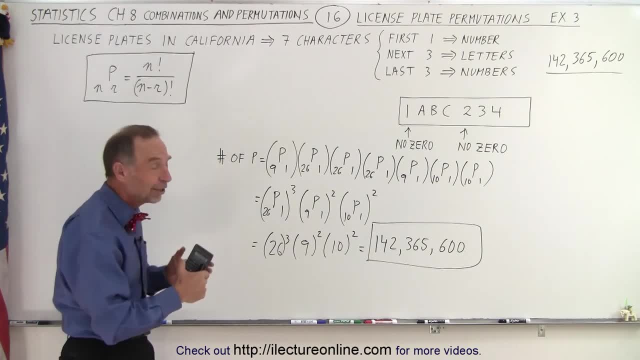 scheme again, or we may need to add- excuse me, add- another character and go to eight characters on the license plate. wow, that seems like a lot of numbers, but it wasn't enough. so let's see how many more we get by changing the scheme and making that first character a letter. 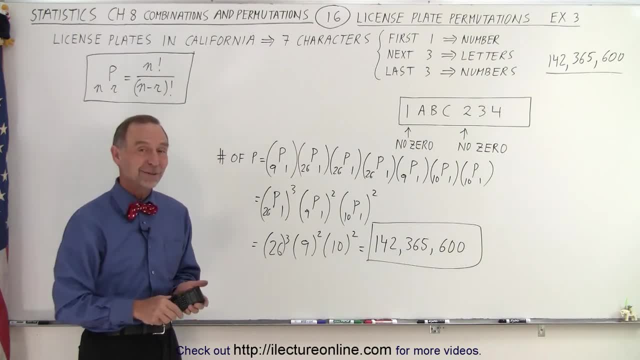 as well as well as a number, and that is how it's done. couldn't they just have flipped the groups of letters and the numbers around? they could have, they could have moved. so what they could have done? they could have moved the letters over here and the numbers over here, and that would